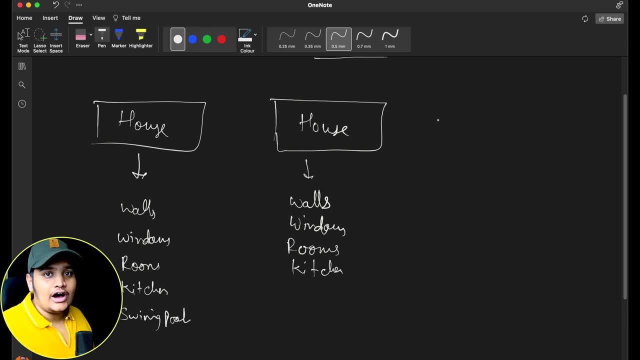 swimming pool as well. And suppose someone tells me that I want a house which has more properties or more features as well. So suppose I want to have the house as well which has all the things, that is, walls, windows, rooms, kitchen. I. 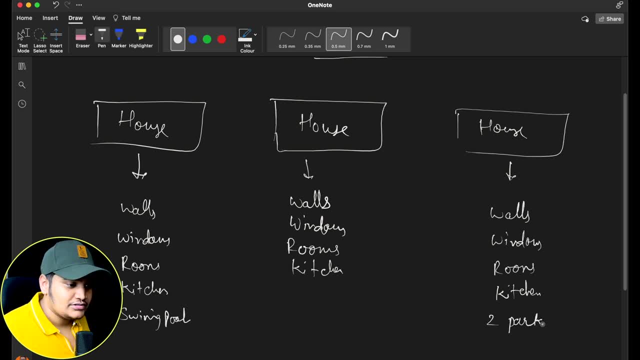 don't want swimming pool, but I want two parkings, suppose, right, So you can see that these are the different features. you can see that someone is asking that I want this particular thing, I want this particular thing. So one thing we can do is: okay, we have the option. 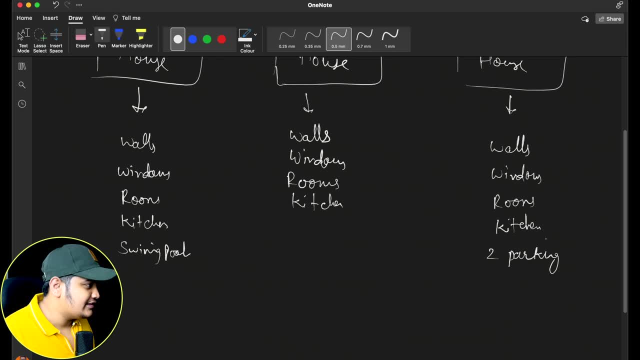 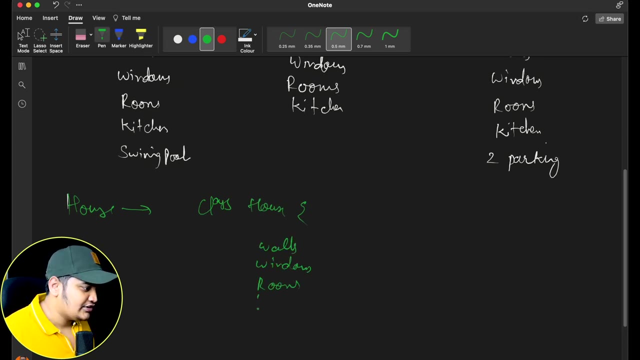 okay to give okay either. what we can do is whenever we are creating the object, we can create the object Right of a house. So suppose, if I'm creating the house object, okay, I have some properties. So suppose, let me create a class house here. I have walls, windows, rooms, kitchen, these. 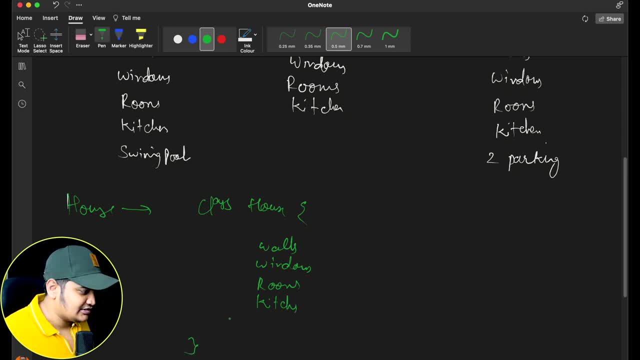 are all the properties right And what I can do is I can have the constructors here, So I can have the house constructor which is taking all these properties: walls, windows, rooms, kitchen and everything. Okay. now someone comes and tells that okay, one swimming pool. 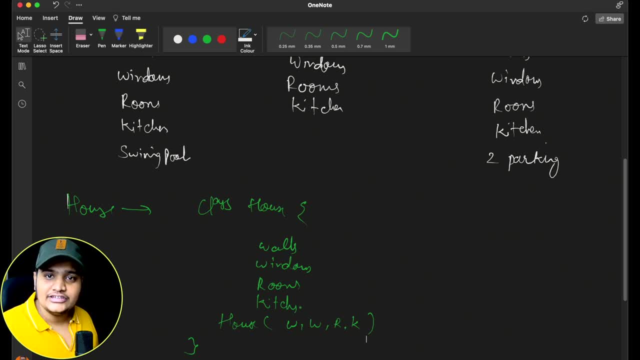 as well. Yes, that's it. they are destroying my house, But the owner did agree. In fact- guess what? they didn't support it. right, My object creation doesn't support that it should have the swimming pool as well. So what I can do is I can have one more constructor I can give House which is taking window. 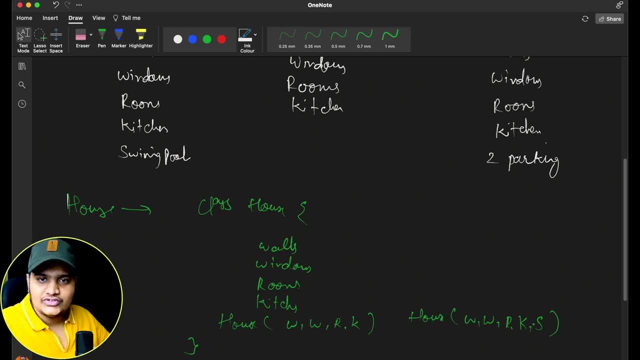 walls rooms, kitchen and swimming pool as well. Okay, so now you can see that my class have the capability to add the swimming pool as well. Now someone comes and tells: okay, I want parking as well. So what I will do is: okay, I will add one constructor that will have the walls windows. 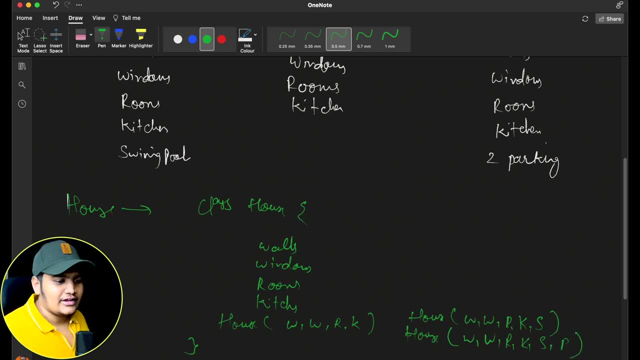 rooms, kitchens and parking as well. okay, so you can see that we will end up with a lot of constructors here right to have the object creation based on the different representation of the same object. okay, so you can see that this representation is different of object, with this representation and the same. 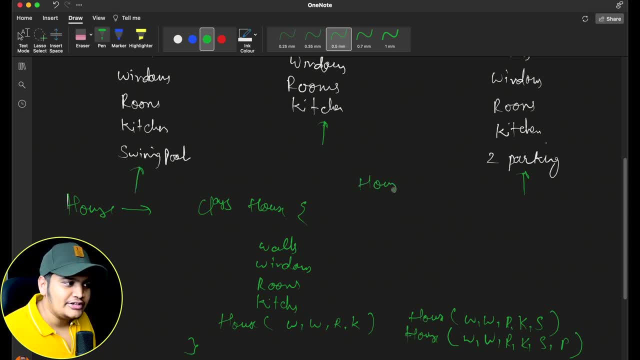 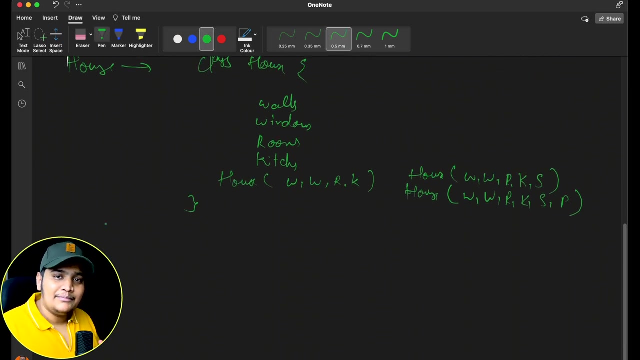 with this representation. okay, all the objects are house object only, but the representation is different. what are part of that particular objects are different. so if you end up in this type of scenarios, at that time we will use the builder design pattern. now, how builder design pattern will help us, so builder design pattern will help us in such a way that, whatever the objects or 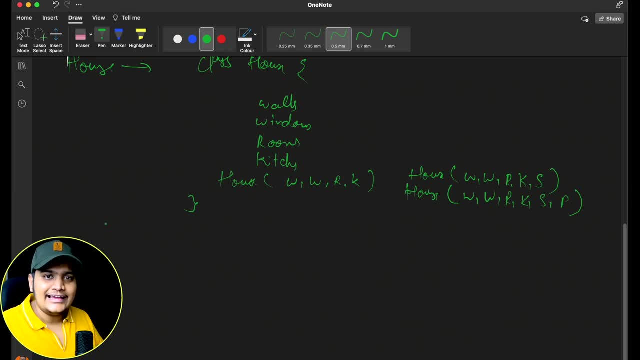 whatever the properties or features we want to add, we can assign those and it will help us to create the object of it, okay. so if i create the house object- okay, this is a class house and what i will do- i have all these properties. okay, we have walls, windows, rooms, kitchen. 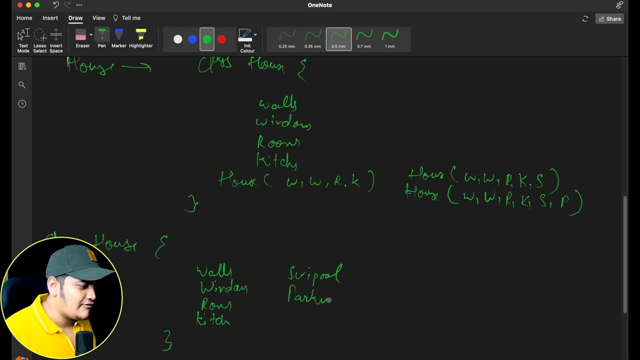 we have swimming pool, we have parking as well. okay, everything we have as a different features or different properties here, and what we will do is we will also provide one builder class. this builder class will be the inner class of the house class itself, which will help to create the 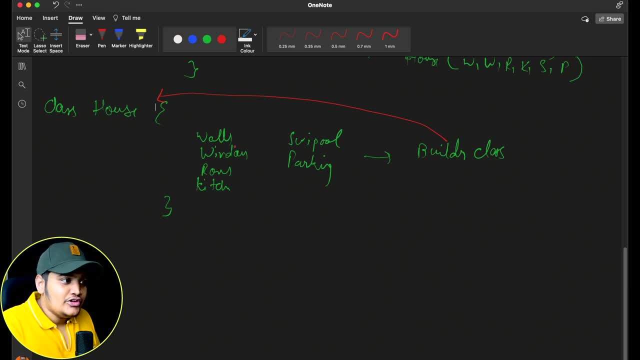 object. so, rather than passing everything in a constructor itself, what we will do is we will use the builder class to create the object. okay, so what we'll do? we will use house builder. we will create one class that is house builder. okay, and within this house builder, what we will do is we 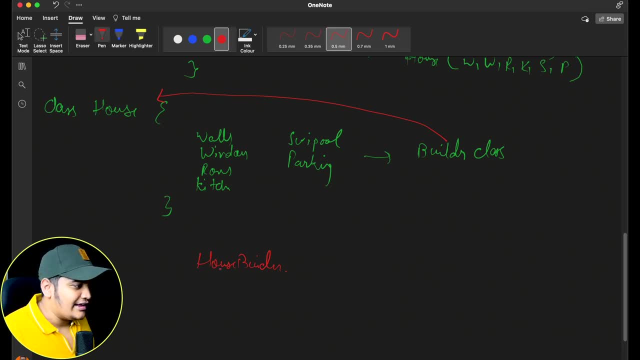 pass all the things. suppose, if i want to add walls, so we will add house builder dot walls. we will have one methods to add walls and we can add walls. how many walls we need? suppose four walls? okay, we have whatever the properties we need we can add. okay, we can have one more method, that is. 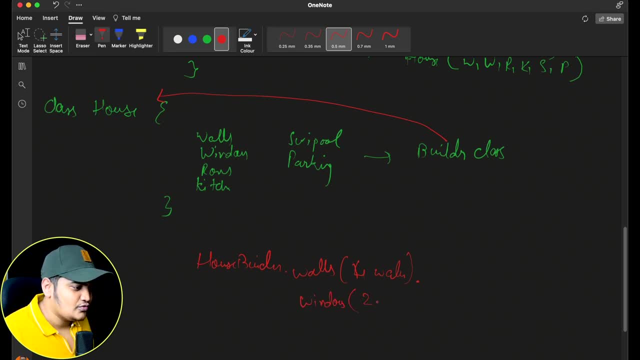 the windows. so you can see that we have the option to add windows opposed to windows. one more method we can add: to add the swimming pool. okay, one swimming pool. we have the method to add the parking as well, so we'll add one parking. okay, you can see that all these different methods are that. 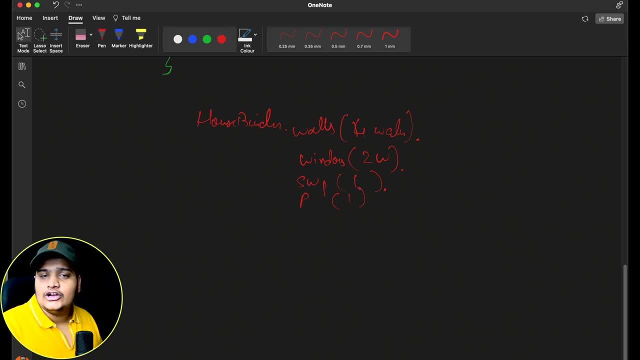 with those different methods, we can assign things like what i want to have in the house, so you can see that this is just a part of the house, builder, and whatever the features you want to add, everything you'll be adding and at the end we will have one method that is a build method, and this build method. 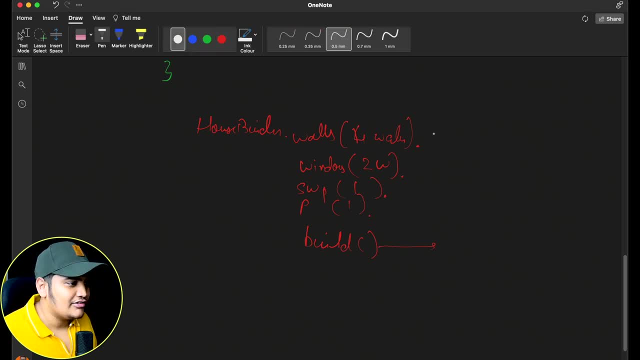 what it will do is, whatever the values are assigned here, okay, whatever the features are assigned here, it will take everything and it will return the house object. so now we are not forcing client to add each and everything in the object creation, so we are not forcing that. okay, if you don't want swimming pool, but still you have to add the swing. 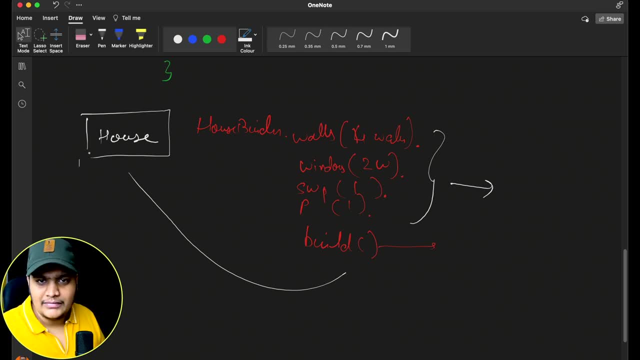 pool, though it's not visible, you can say no, but okay, so we are not forcing that way. we are giving the option to the client, like, whatever you want to add, add those things and we will create the object for you. okay, we will create the product for you. so we are giving control to the client itself, okay, so 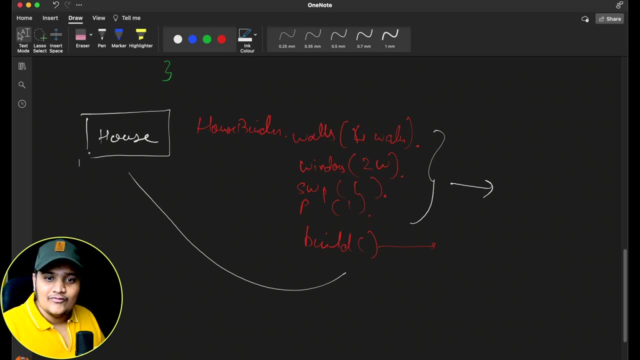 that's why you can see that the step by step creation they can do with the project creation, with the different representation of the same object. now suppose tomorrow they will come, okay, they will use this house builder and they will not add anything and they will directly call the build. 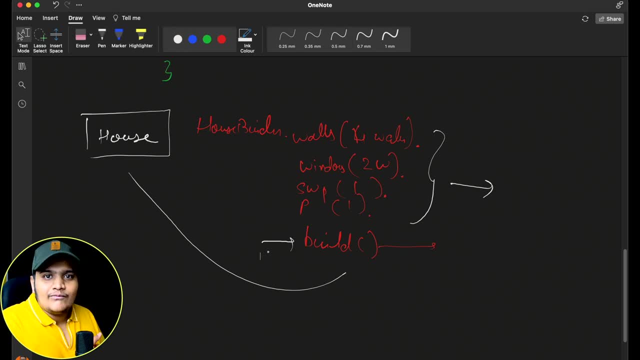 object: okay, but you need some basic properties, right, you need some walls, windows and everything to have the base house ready. so for that, what you have you can do is, whenever there is a build method called, you can have those validations as well, like: these are the basic things that you need. 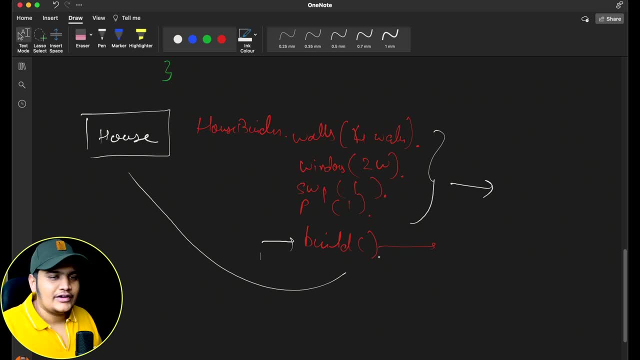 to add while creating the object of it. okay, so those validations also you can add. so this way, you will provide the base properties like this: we are going to have what we call the build object, basically all the objects, and we need to offer this slide as well, which you can add. that is today the 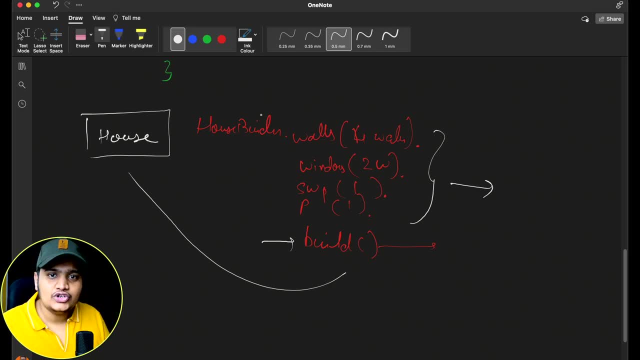 beginning of the world. showing will be a little spoiler of this video. usually you can add: but this way 100 years is No show. this and then. hopefully you enjoyed this episode of the process. so if you enjoy watching our video, comment and properties should be needed to create the object and you will give the option to add different. 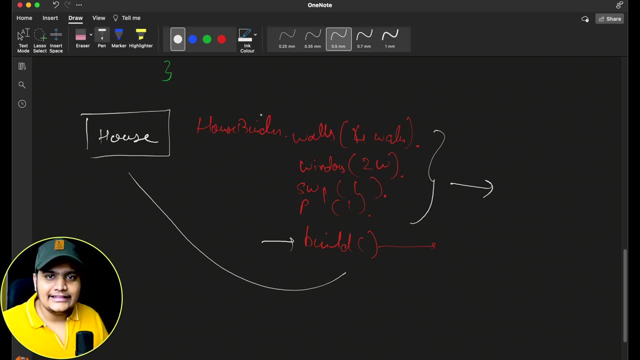 properties based on that requirement itself. We are not forcing anything to the client, like you have to add each and everything. Okay, so this is the basics of the builder design pattern and where we have to use the builder design pattern. Now let's understand the same thing with the code. 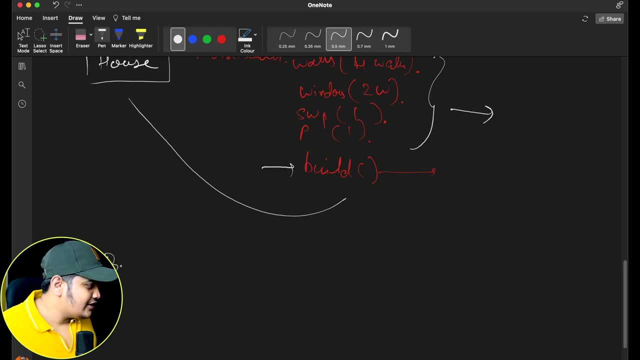 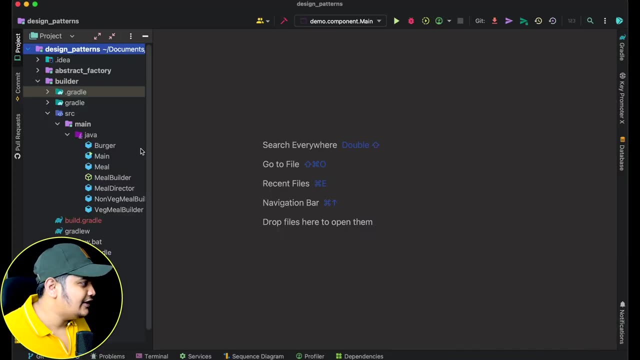 So in the code we have taken the example of a burger, okay, where you can create a burger with the different ingredients in it, right? So let's understand that. So let me go to the example here And you can see that I have created one burger object, Okay, so this is the burger class, And 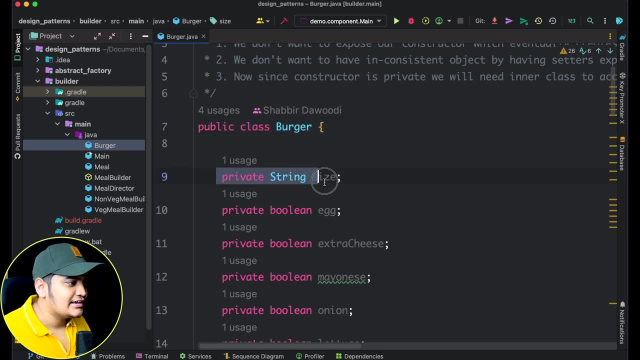 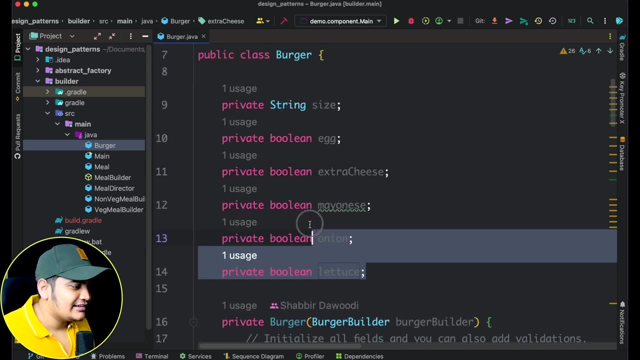 this burger class have these properties. you can see that it has the size of the burger, eggs, extra cheese, mayonnaise, onion lettuce, etc. Okay, so you can see that these are the properties that they can assign. okay, user can use to create their own burger. simple thing, Okay. 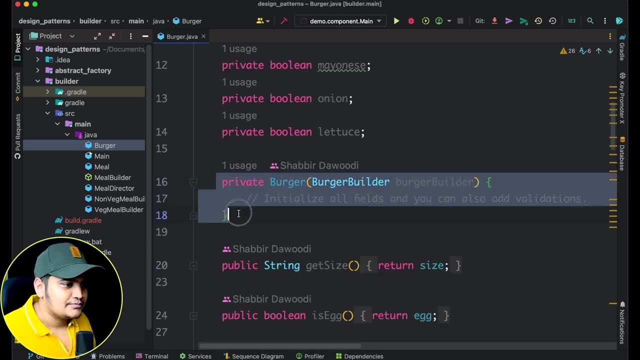 Now you can see that this is a constructor here. Okay, now you can see that this constructor is taking the burger Builder as the input parameter, And here I mentioned that this is to initialize all the fields and to do the validations. So, as I explained you earlier, like whatever the validations we have, 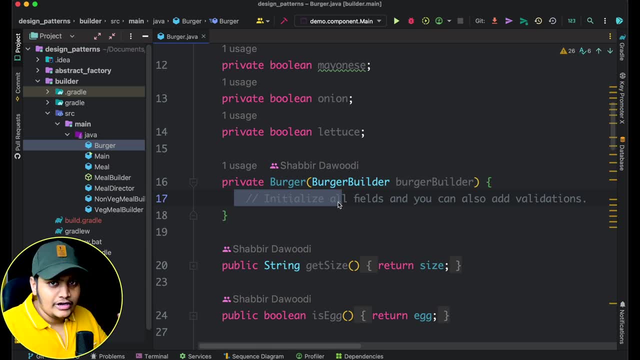 to do, like all these basic properties you need if you want to create a burger, you need to have the bread itself right. Without the bread you cannot create the burger. So all those types of validations we can add here, like you need all these properties, If these properties are not. 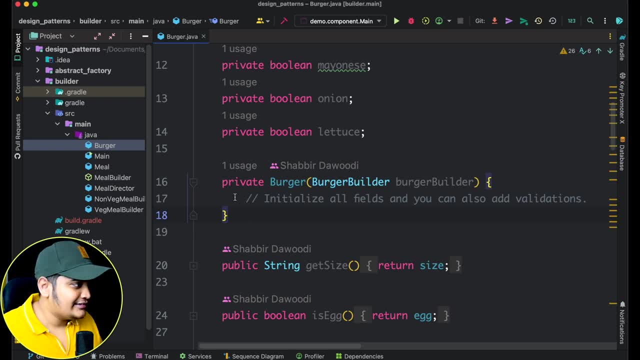 there you can throw the exception. So this is the constructor that we have created, And you can see that this constructor is private. Okay, so user will not be able to call the constructor, But the burger builder class that we are going to create that will use it And, as I explained, you, 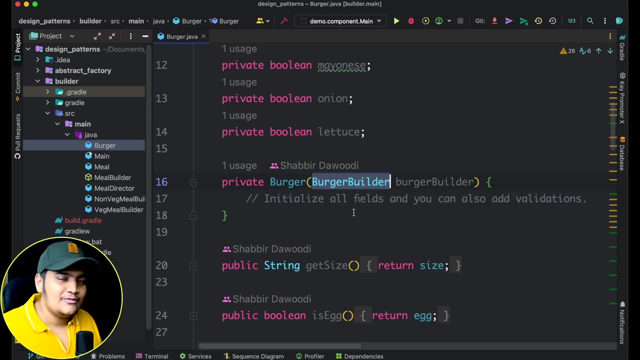 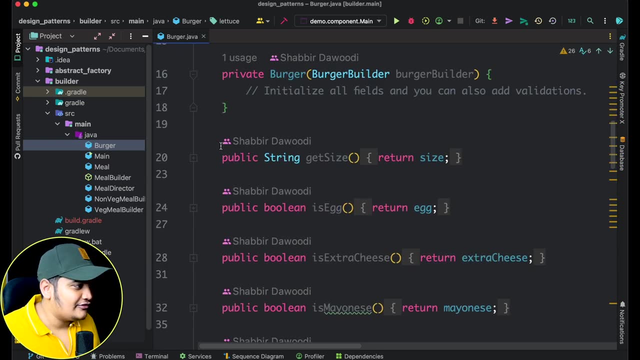 earlier. whatever the builder class would be there, that builder class will be creating the inner class itself directly. Okay, So you can see that, for all this fields that we have, for all that fields, what we have done is we have added the values here, we have added the getters, all the. 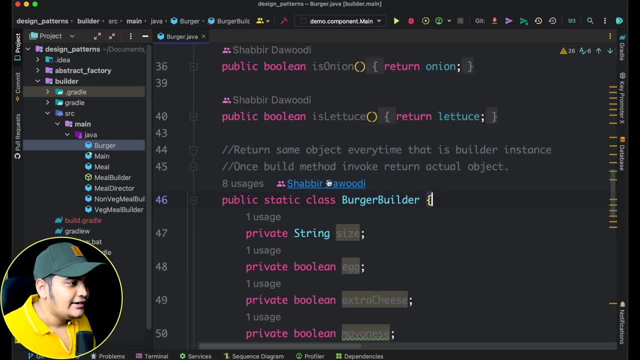 getters method. we have added here: simple thing: no setters. Okay, now you can see that we have created one public static class, that is the burger builder. Okay, so this is the inner class, inner static class, So we can directly use this. Now you can see that we, within this class, 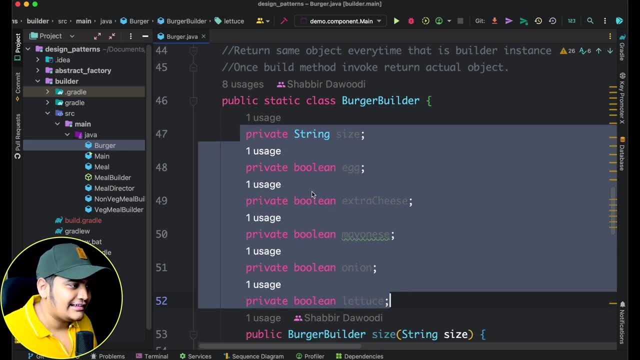 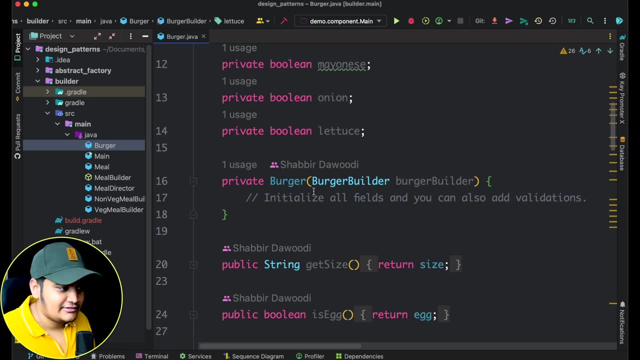 we have added the same properties here. Okay, you can see that these are the same properties that we have added in the burger class itself, because we will use that to set the burger properties. Now, all these properties are there. Now, you can see that to set all these properties. 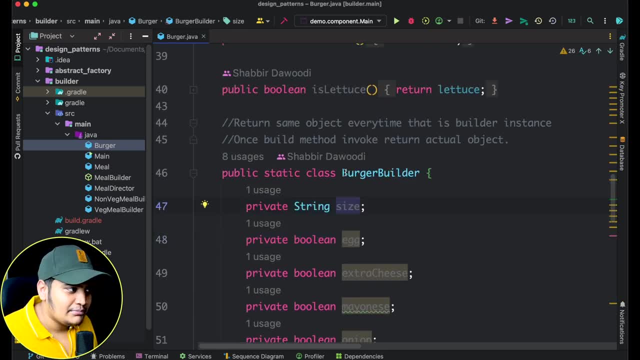 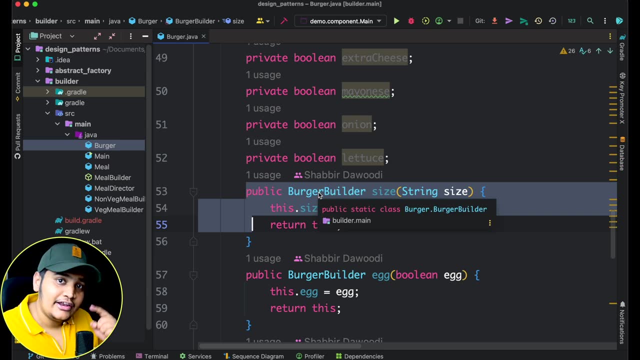 we will be using one method that will return the burger builder itself. Okay, so to set the size, you can see that we created a method that is public. It is written in burger builder itself And it is taking the size and we are setting the. 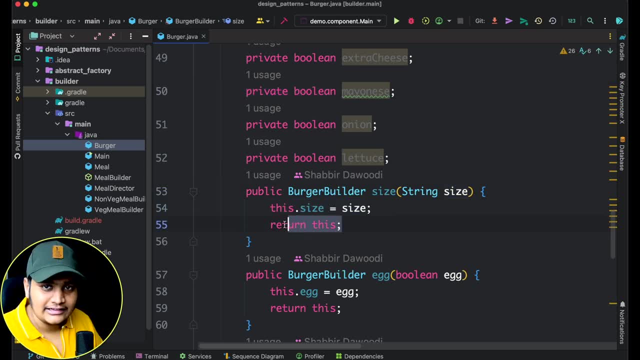 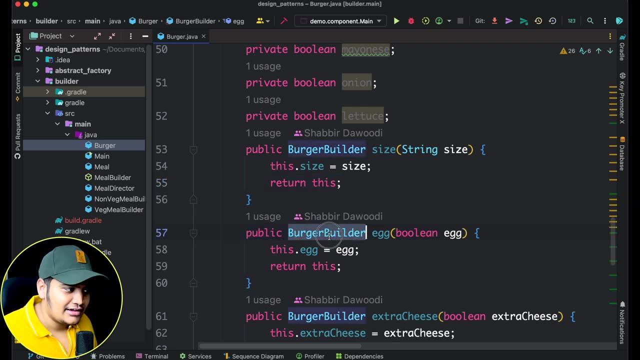 size within this class And we are returning this object itself. we are in the same object, that is the burger builder. Similarly, for setting the egg, we are having the same method. that is the burger builder. it will return the burger builder, it will set the eggs and it will return the same. 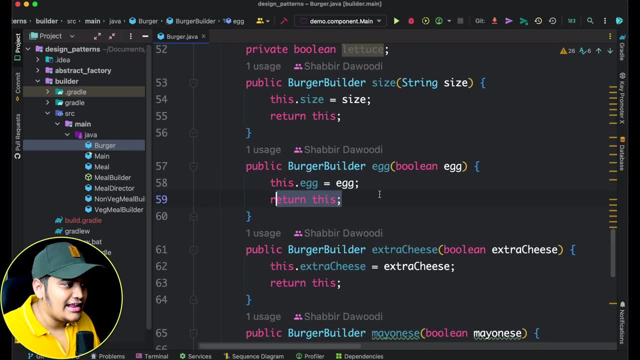 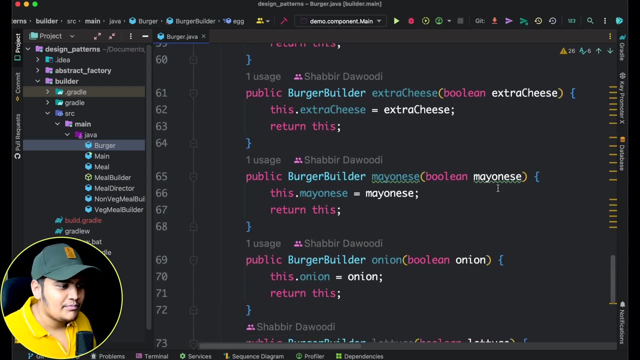 object for each and everything. to set all those things, we will have one method that will return the same object itself by setting the values: Okay, eggs for extra cheese, for mayonnaise, for onion, for lettuce, etc. so all the things are set. now, once all. 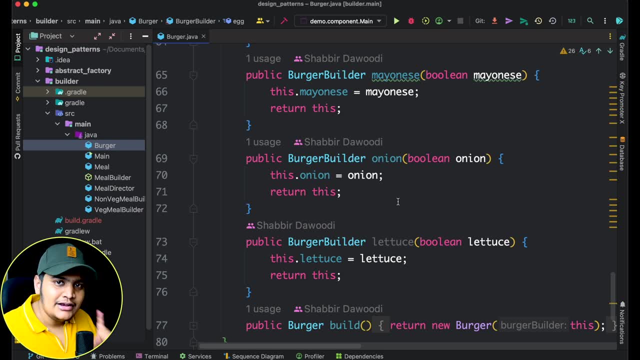 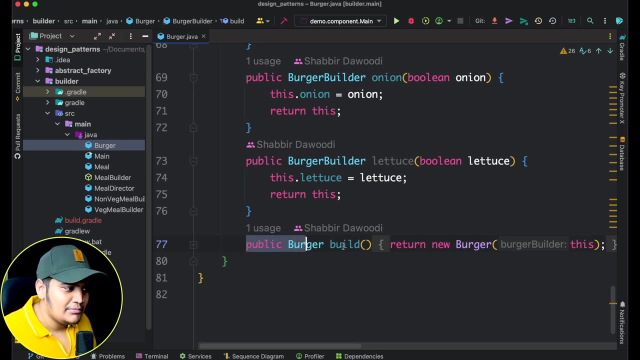 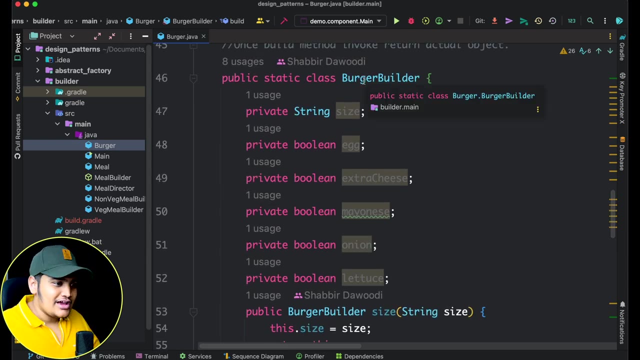 the things are set, we will have one method that is a build method that will help to create the entire object for us. okay, so here you can see that we have one method that is public build method, which is going to return burger. okay, because this you can see that this is the burger builder. so we are. 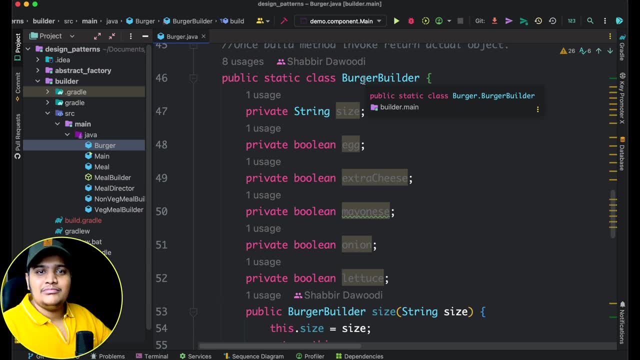 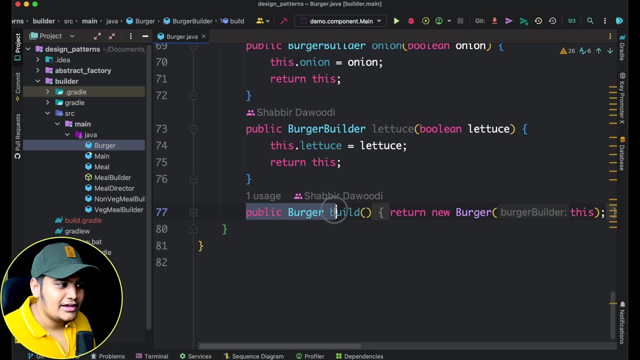 building our burger and at the end, we have build method that should return me the burger, because that's the end result i want. so once we have this method created, that is, public burger build, you can see that what is returning here, it is returning new burger and the object: 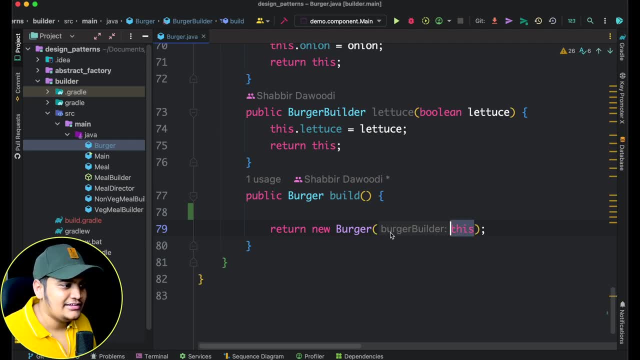 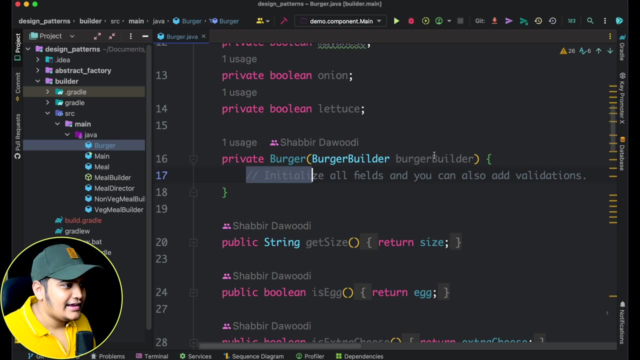 that we are passing. is this, okay? so the input is this object, that is the burger builder. now, if i come here, okay, here what i can do is the entire burger builder is coming here, right, so here i can do all the validations. okay, and all the validations are done here or not. 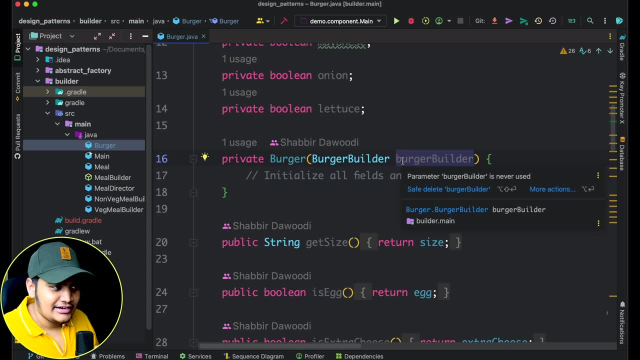 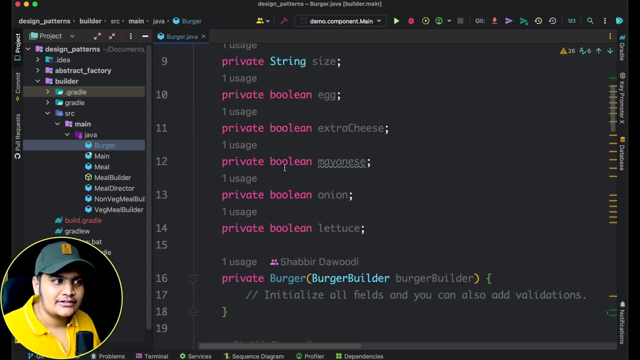 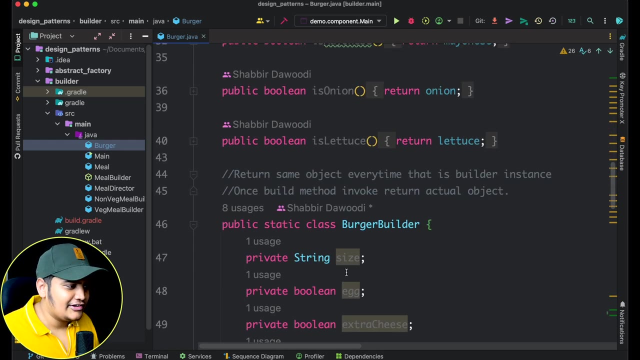 okay, if all the validations are done and everything is there, what we need, then we can assign all those values to this object, okay, and return this object. simple thing, okay. so whenever i want a burger, i will use burgerburgerBuilder, then i will set all these properties and it will call the build method to build my object. 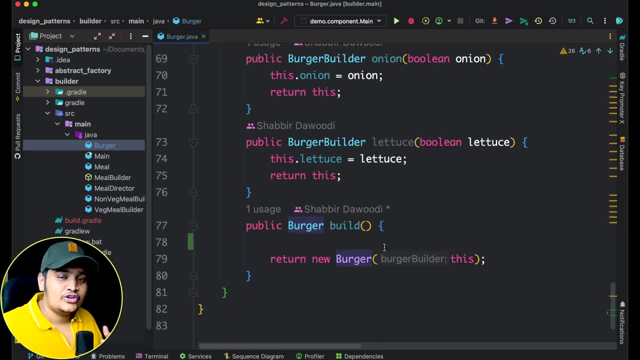 so this is the simple way you will create a builder design pattern. so now, if you are aware about the ganso 4 design pattern book, in that there is also one extra thing mentioned, that is the director. okay, so let's understand that part as well. so here you can see that. 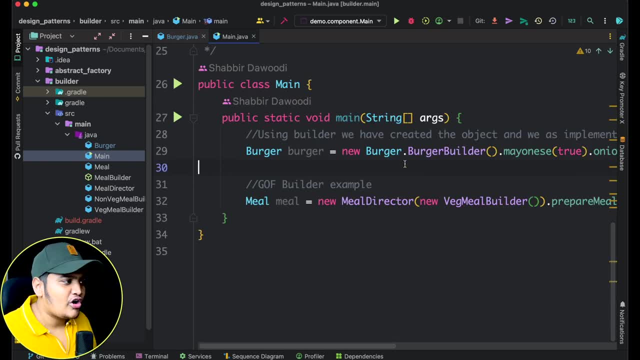 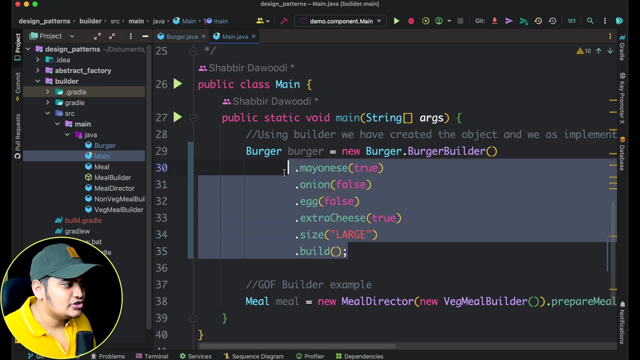 in the main class if i go here. okay, you can see that how i will be calling this burger is so burgerburgerBuilder. i will add mayonnaise, i will add. you can see that i am adding all these values here. right, and at last i am calling the build method here. okay, so this: by setting: 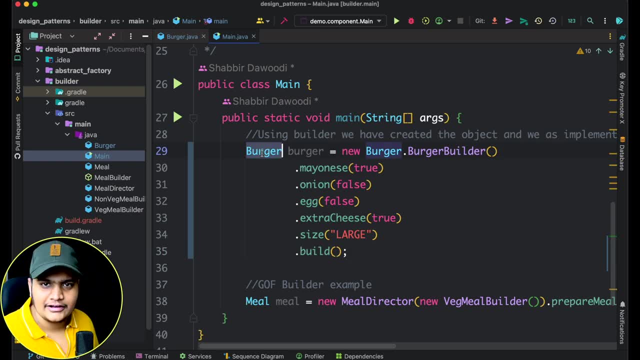 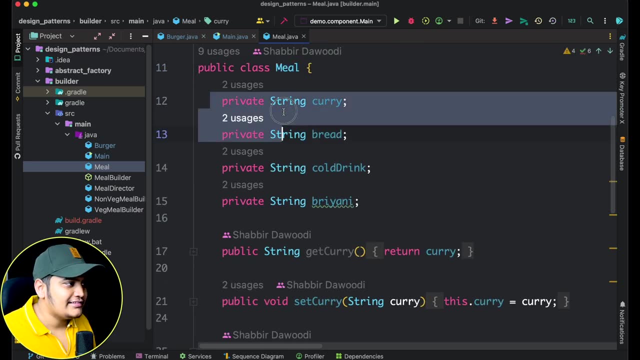 all these values and by calling the build, it will give me the burger here. now let's understand about the director as well, okay, so here you can see that i have a meal object. so meal object has few of the properties, that is, the curry, bread, cold drinks, biryani, etc. and these have the gatters and setters as well. okay, 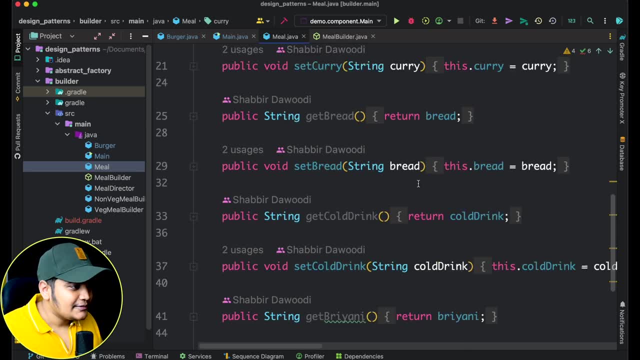 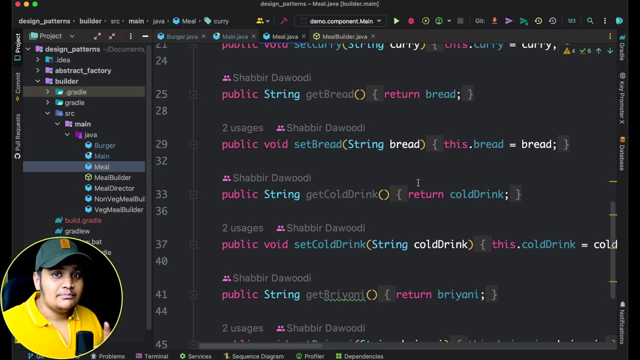 simple meal object. so you can see that for this meal object, okay, we have all the gatters and setter's, everything set. now this meal should also have a builder with which we can create the object. but meal- we can also be a veg meal as well and a non-veg meal as well. 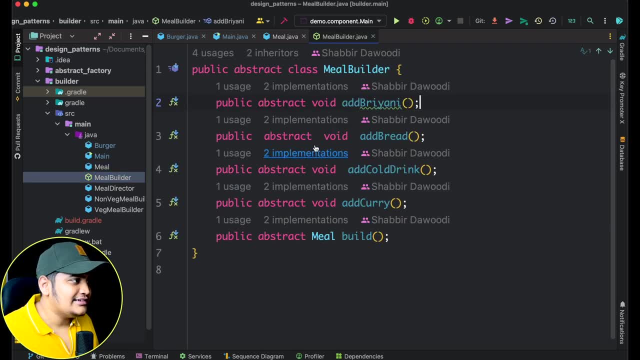 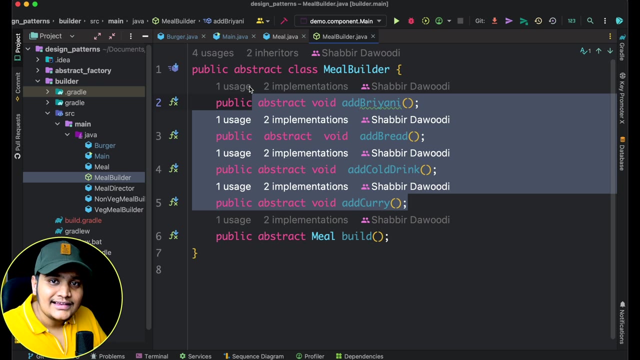 okay, so if i go here in a meal builder, you can see that this is the abstract class and this abstract class has all the different abstract methods. okay, so you can see that it can have add biryani, add bread, add cold drink, add curry method. okay, all these methods are to add the basic. 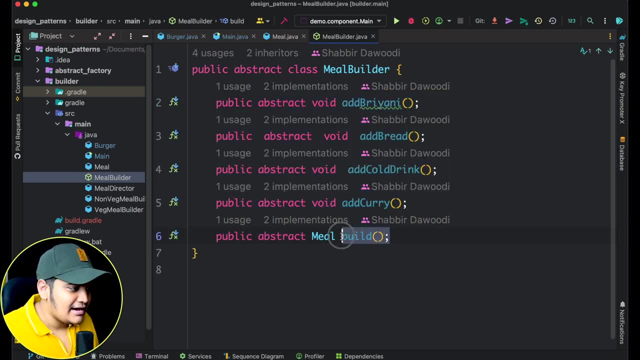 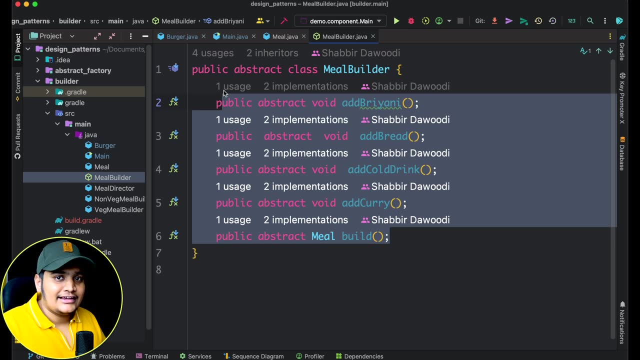 things of a particular meal and it has a build method which will return the meal as well. okay, so all these abstract methods we have defined here, now we can have the multiple classes, that is, the veg meal builder and a non-veg meal builder. that two class should. 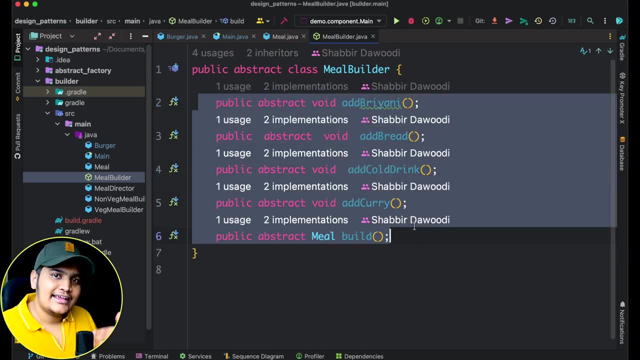 implement this abstract methods so based on that, they can assign the values. okay, so they can create the object either. if we pass veg finden veg brain, it should create the meal which is veggies meal. if we provide non-veg builder, it should create a non veg meal. okay. 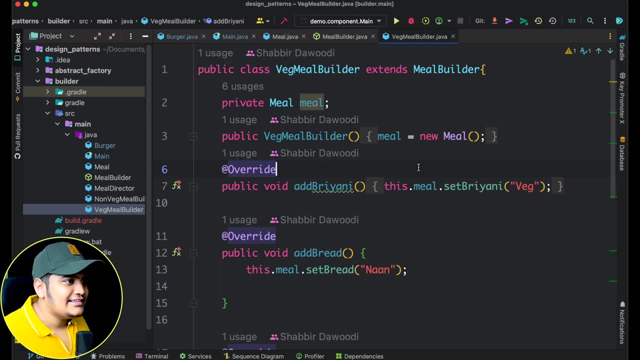 if I go to this veg stress builder, you can see that veg meal builder is also extending the meal builder which we have already defined yet. so once we extend this, we have to add the implementation of all the abstract methods. So here you can see that veg build and veg. 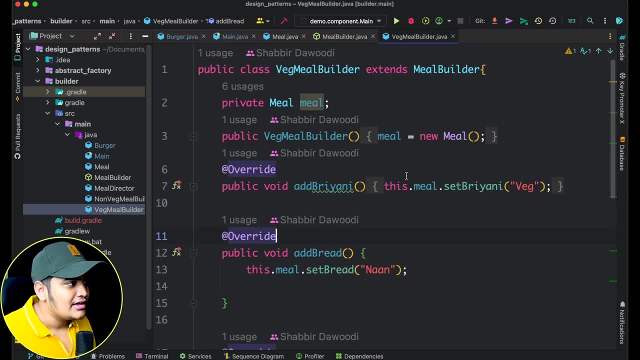 beader, have implementation of all the abstract methods, okay. but here one thing: you can see that we have the object of a meal itself. okay, because from the veg builder, we want to return the meal at the end, right, so that's why you can see that it's going to return the new meal, okay, from this constructor. 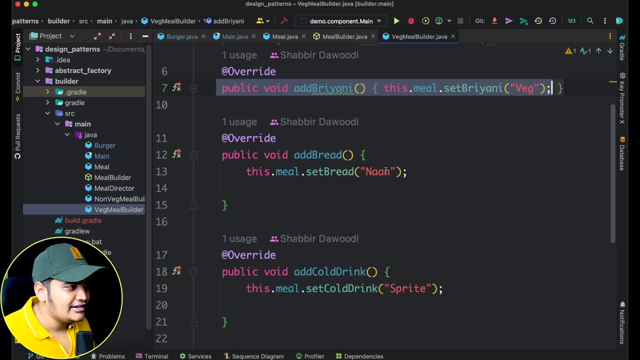 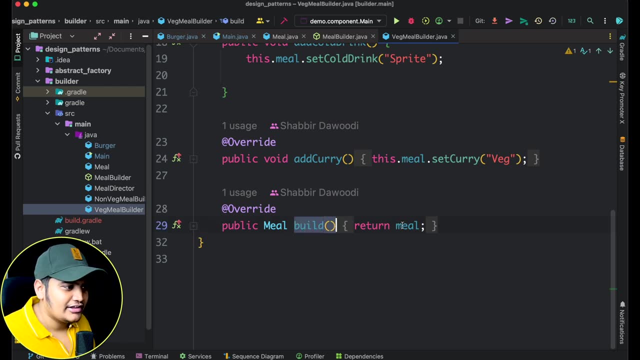 now all this method. you can see that add biryani: is adding the biryani, that is veg biryani. add bread: is adding the naan cold drink. it's adding okay, curry, it's adding, and you can see it has a build method which will return the meal object. similarly, if you go to the non-veg meal, 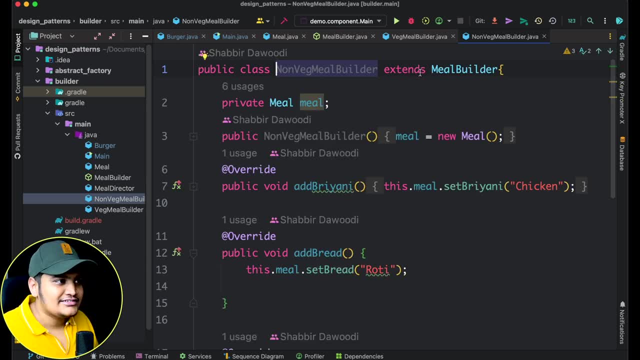 builder. we have the same thing. non-veg meal builder is also extending the meal builder and it has the meal object and it is going to have all the methods similar to what we added in the veg meal, but the values would be different. okay, so you can see that now you have two builders. 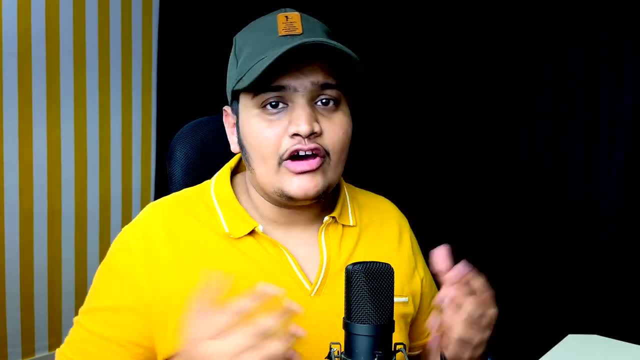 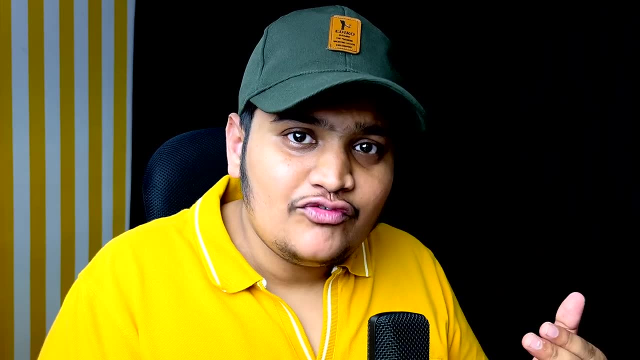 available. that is, the veg meal builder and a non-veg meal builder. now, as i have two different types of milk created, that is a veg meal and a non-veg meal. whenever any customer asks: okay, i want a veg meal, so by default i should have something that goes based on the value veg and gets all the veg item only. 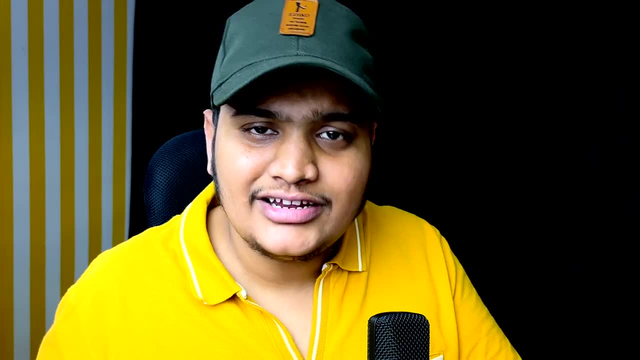 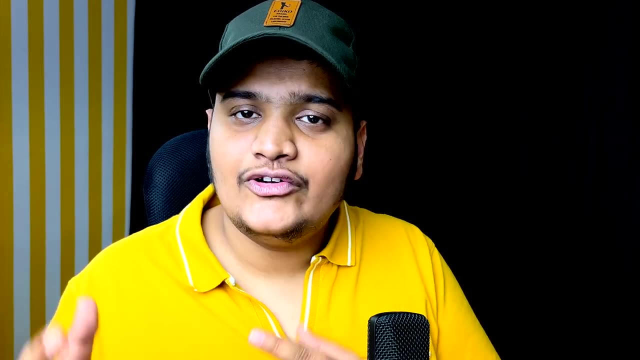 so it will create each and everything. it will add each and everything in a particular object and it will return me. if someone says that i want non-veg meal, okay, it will add all the non-veg items and it will create a meal and it will give me that. 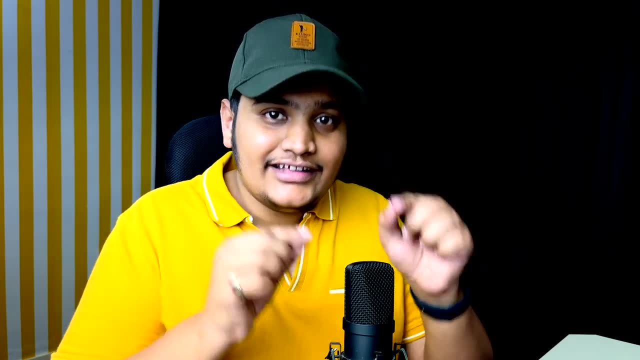 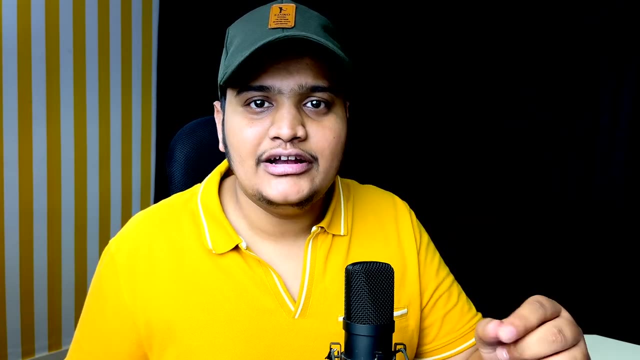 particular thing. what i'm talking about that's called the director. so that director will take the input okay and based on that input it will go call a particular builder and that builder will return the particular meal. similarly, if i ask the director that i want the non-veg meal, it will. 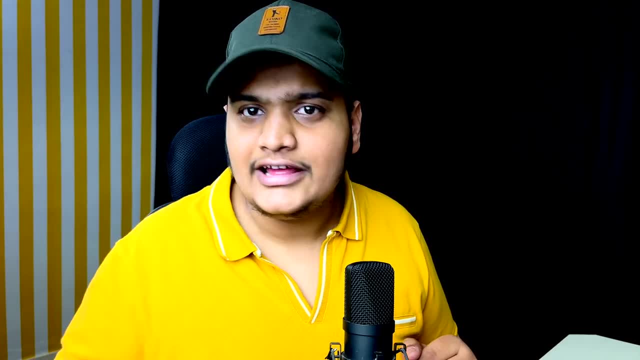 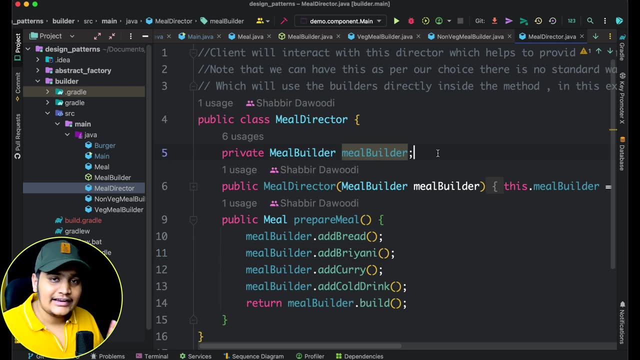 go to the knowledge builder. it knowledge builder knows that what we need to add and it will add everything and it will give me the object. okay, so that's the job of the director here. so if i go to the meal director here, you can see that mail director has the object of a meal builder. so 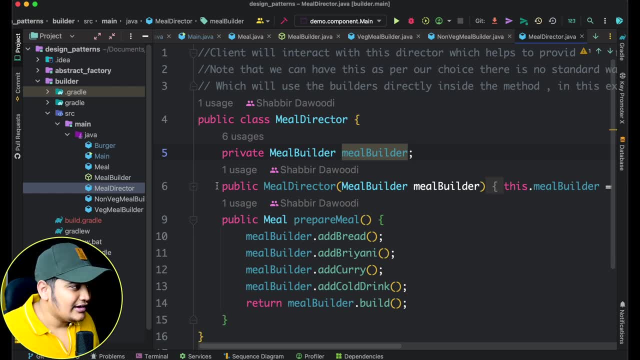 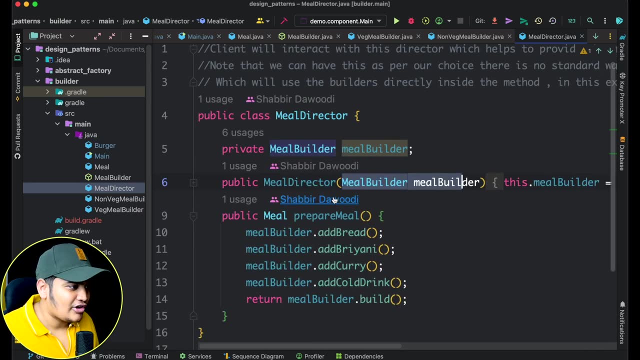 it knows that what we need to add so you can see that mail director. okay, there is a constructor here and this constructor is taking the meal builder object. okay, and within this meal builder method, it is calling all the methods: add biryani, add bread, curry, cold drinks, everything and at. 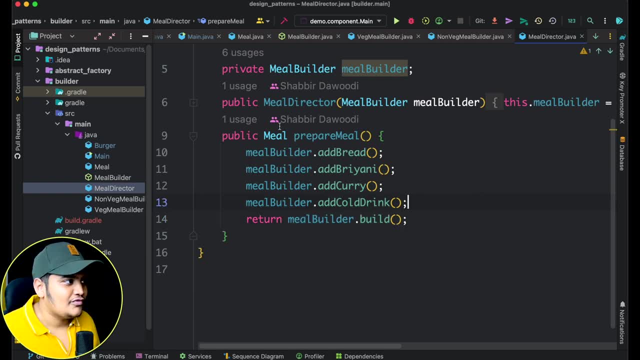 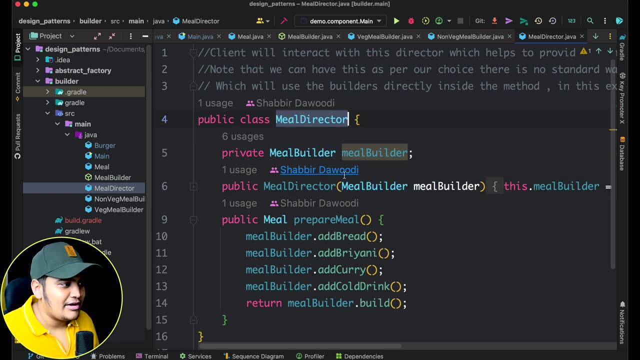 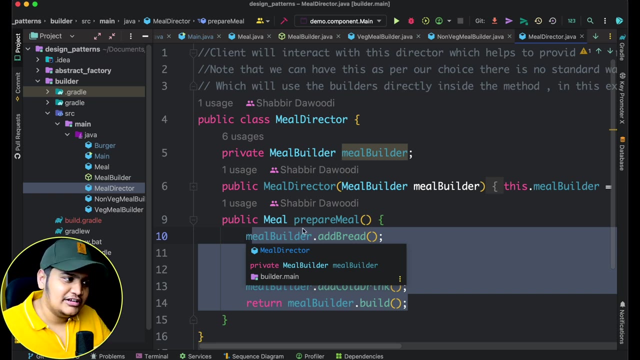 the end it is calling the meal builder dot build method. so whenever i will call meal director here and i will pass the proper builder here, suppose in the meal director, if i pass wedge builder, it will call all the methods of a wedge builder and it will create the meal which is a wedge meal. 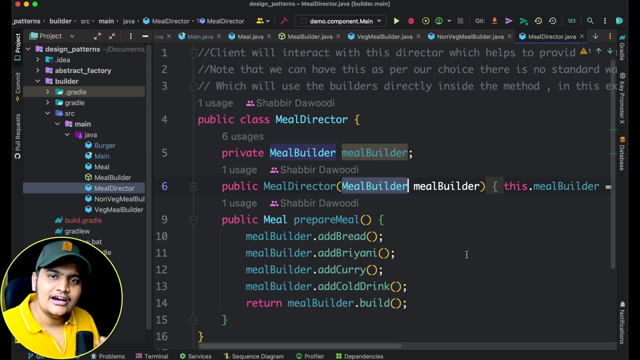 if i pass the non-veg builder, it will add a non-veg items and it will give me the non-veg meal. okay, so you can see that that's the part of the director here. so whenever i want to call it, if i 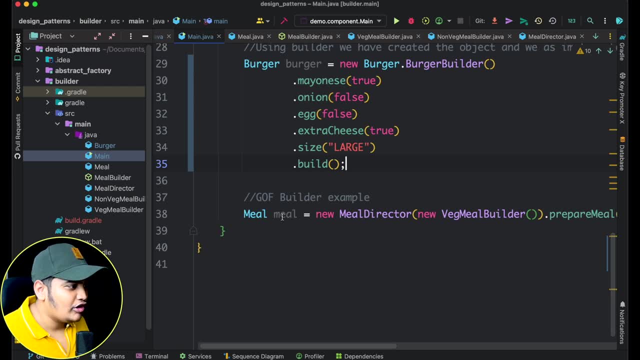 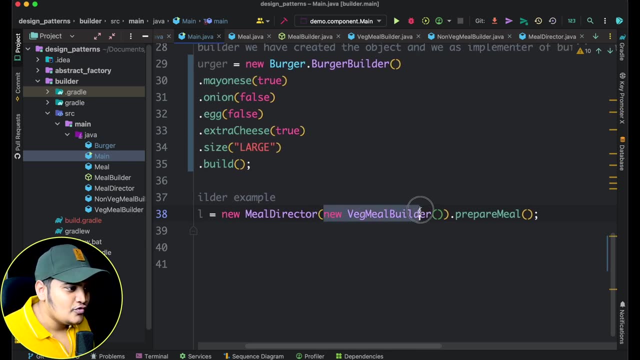 go to the mean. you can see that how i'm calling. i want a meal, okay, and i'm calling the meal director, so in the meal director i'm passing that. i want a new wedge meal builder, so i'm passing the new wedge meal builder. so this is something that it will return the wedge meal and that's why.